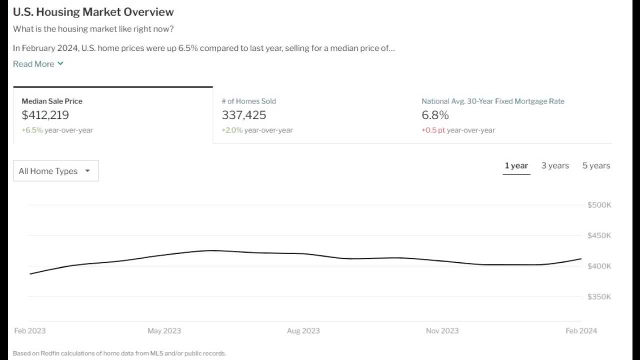 month. Since the previous month, home prices went up by $9,696.. Are homes still unaffordable for millions of Americans? Are homes still affordable for millions of Americans? Are homes still affordable for millions of Americans? Are homes still affordable for millions of Americans? Are? 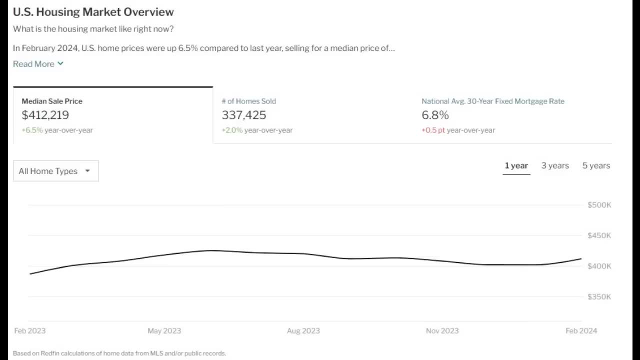 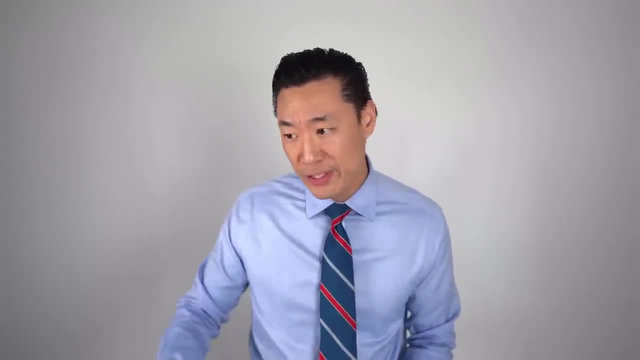 the answer is yes. Has there been a housing market crash? No. Now I want to remind everyone that this is the median home price in the United States of America, So I understand that there's going to be people in the comments saying that in my area home prices are down by 20%. 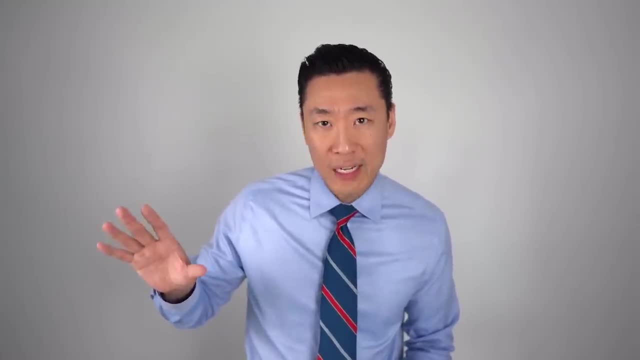 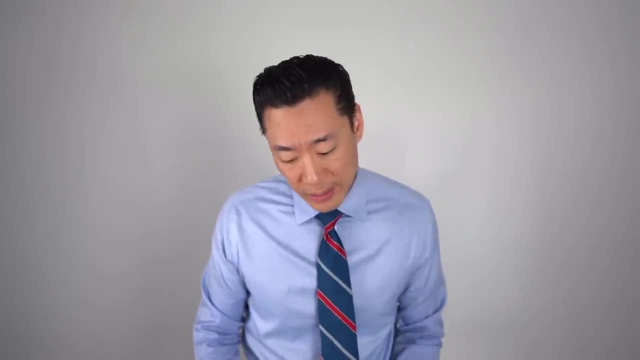 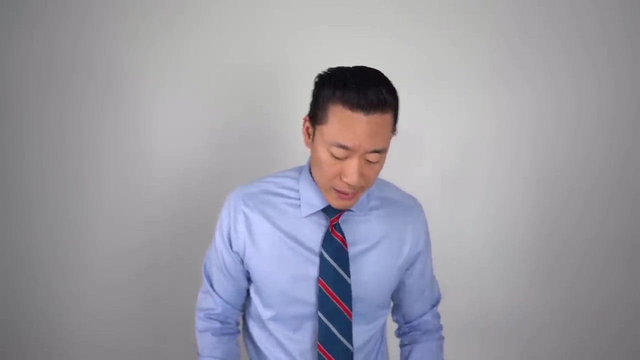 I'm not going to deny that. But if home prices are down by 20% in your area, that means that home prices are up by 26% in a different area. If you don't believe in math, then what can I say? I'm not going to argue with you. Okay, now I want to tell you this. I know that. so 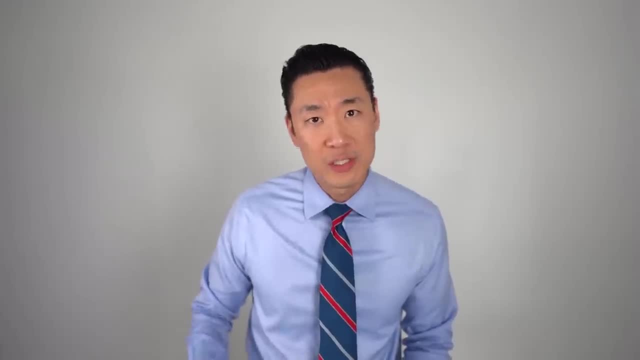 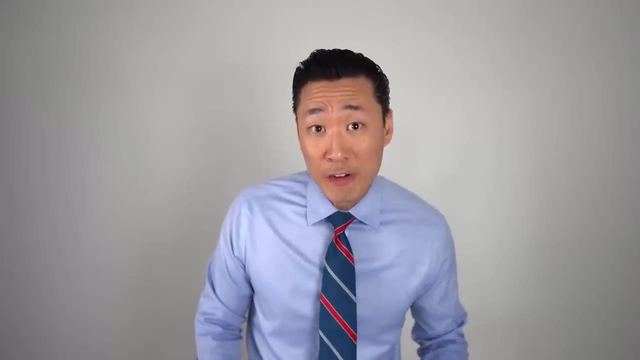 many people have been saying that there's going to be a housing market crash. It's coming, It's coming. They've been saying that for the past three years. So listen, I get it. Housing is unaffordable, right. We want to see some relief, but it's just not happening. So this is what 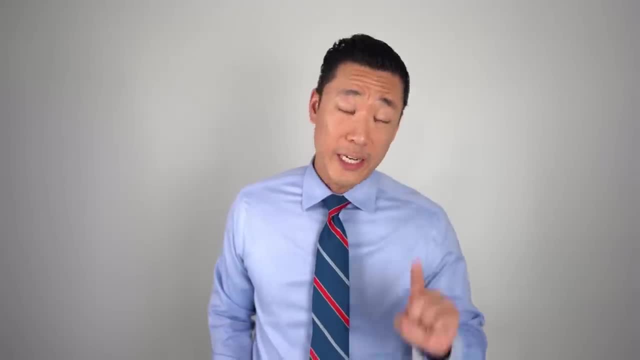 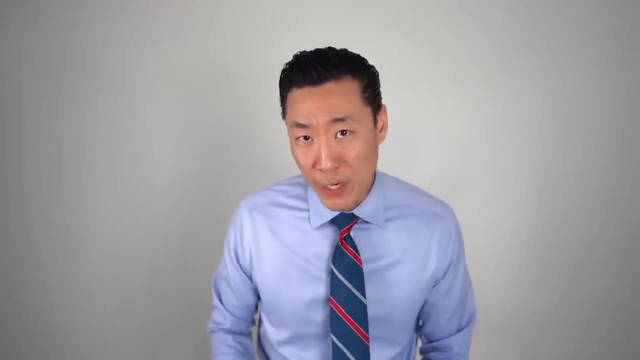 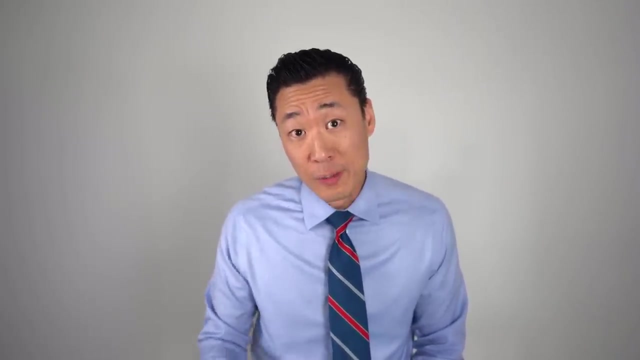 happens when inflation gets out of control. Okay, you have to hear this one because I don't know if people picked up on this. There are some scary developments going on right now and I think it's just going to get worse. If you were paying attention to the Federal Reserve press conference. 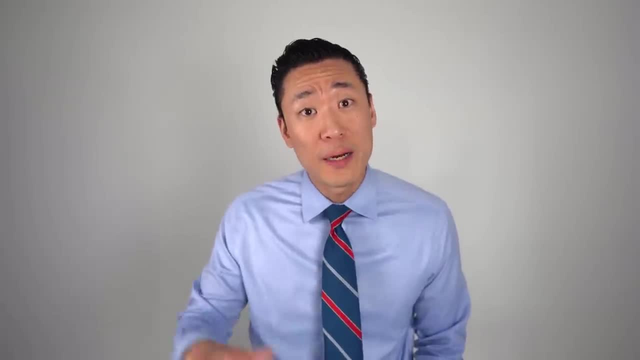 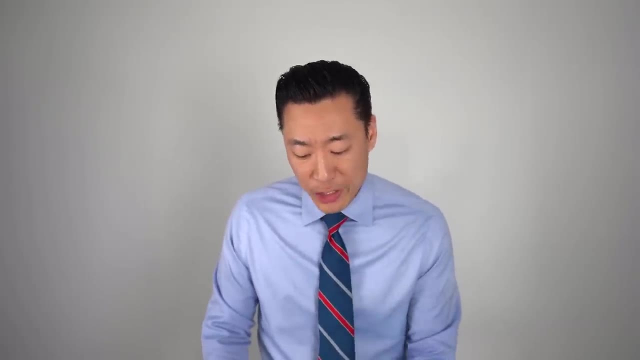 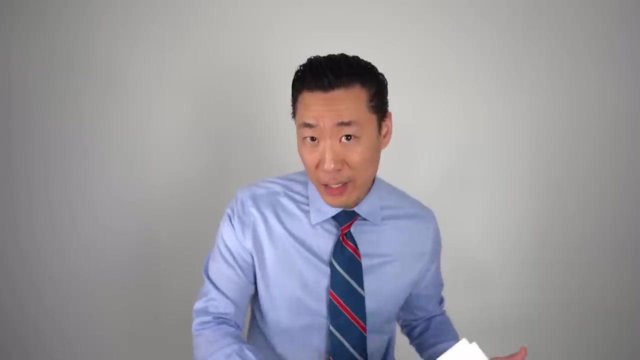 the most recent one. So Jay Powell. he spoke about housing, So I don't know if you picked up on this. So Jay Powell is the chair of the Federal Reserve. At the Q&A session they asked him about housing. They were asking about how housing prices are not coming down, how this. 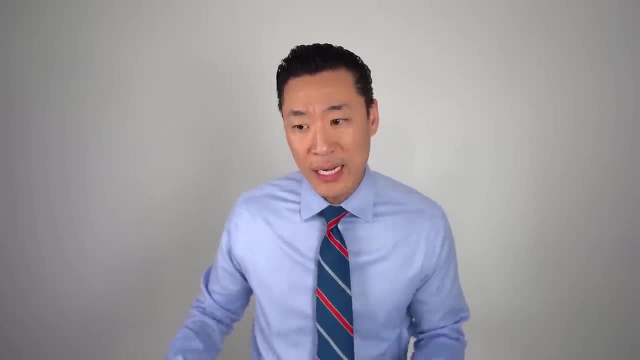 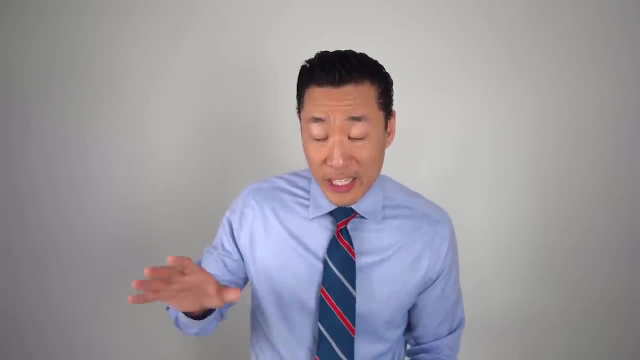 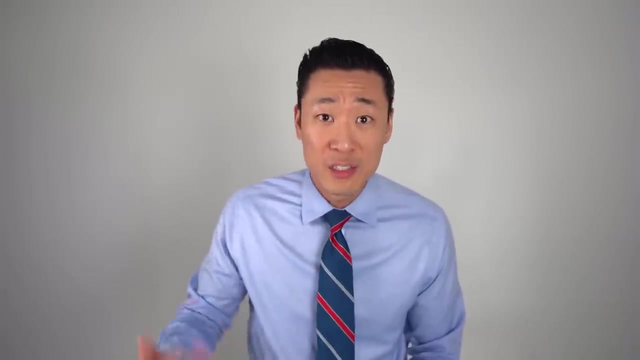 relief that we were expecting, but it's not coming. how it fits into the whole inflation picture. So what's scary is that Powell said that he believes that they can bring inflation down to target to 2%, even if housing doesn't come down. So, ultimately, what Jay Powell is saying- is that these higher home prices could be the norm, like they're not coming down, and I wouldn't be surprised. Another concern of mine: what is the Federal Reserve planning on doing? What's the upcoming monetary policy? It's two things, and it's going to affect housing significantly. They're going to cut interest rates and that's going to lower the 10-year yield and that's going to lower mortgage interest rates. But before you celebrate like yay, mortgage interest rates are going to come down. Before you celebrate, you have to remember, you have to think about it. What's? that going to do to home prices? Lower mortgage interest rates. What's that going to do to home prices? Well, it's going to dramatically up interest rates and that's going to add buying pressure and that's going to send prices up more demands. And you know what I'll be the first to admit that it is a terrible situation. If you keep interest rates high, then you're going to have housing unaffordability for buyers, right, But if you send interest rates lower, then the home prices are going to go up. So listen, okay, it sounds like a case. 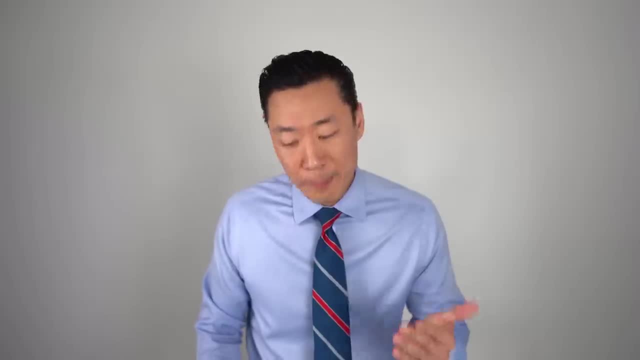 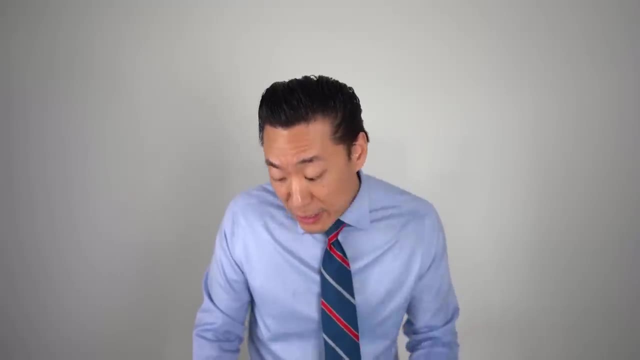 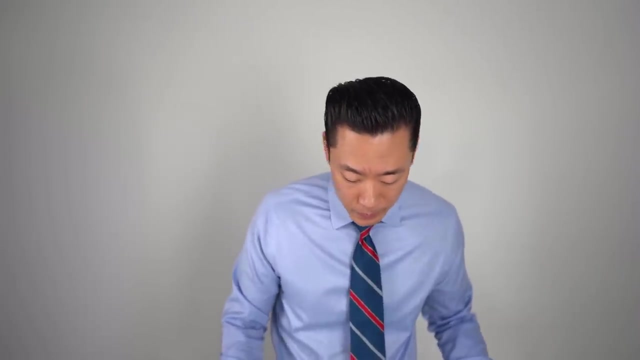 you don't right, But when mistakes are made, people suffer consequences. You can't just make a mistake and nobody suffers. There have been some serious mistakes with monetary policy by the Federal Reserve and we are paying for it. That's what's going on. The second concerning thing is that the Federal Reserve is 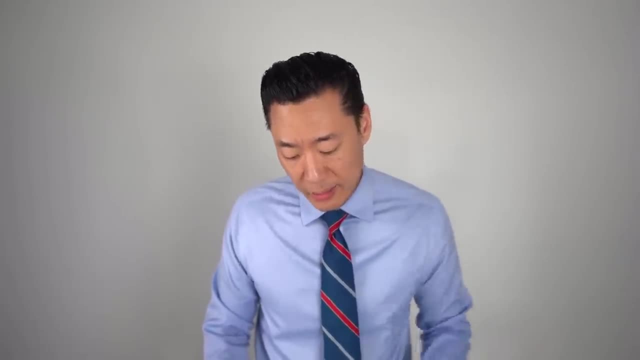 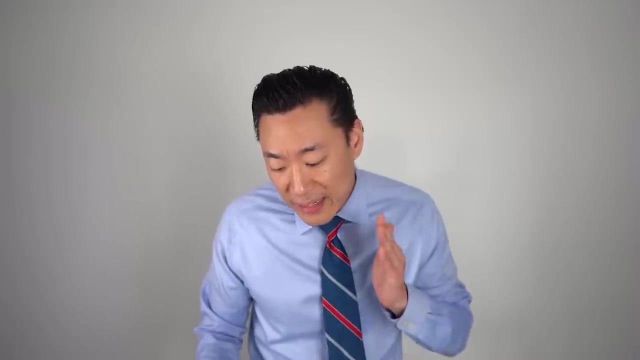 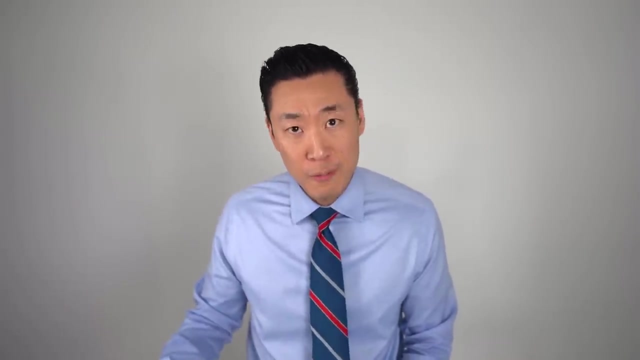 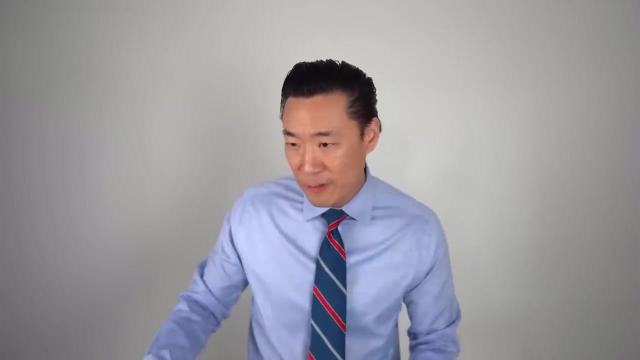 going to switch to money printing again, which is obviously inflationary, And they're gonna start the transition this year and probably soon. They announced a plan to slow QT switch to QE, which is a fancy term for money printing. So the plan, it's public, but they used a technical jargon to hide all of this in. 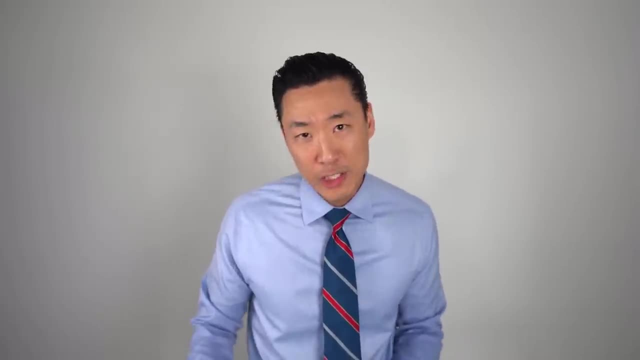 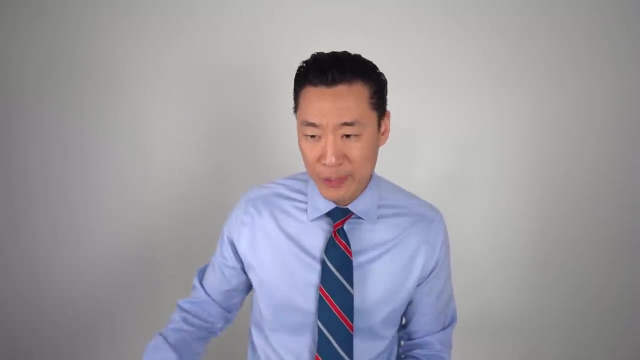 plain sight, But that's what they're saying In layman's terms. they're gonna cut interest rates and they're gonna turn the money printers back on, And you can take a guess as to what's. what's gonna happen to home prices, what's? 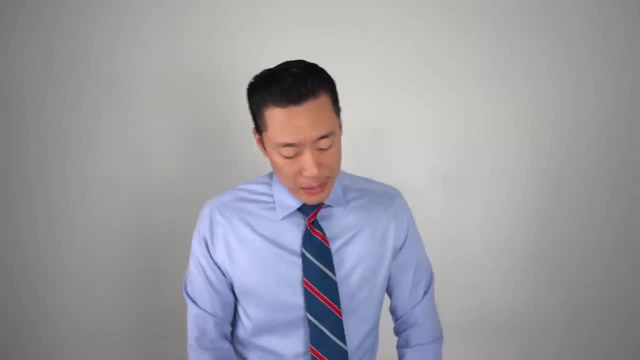 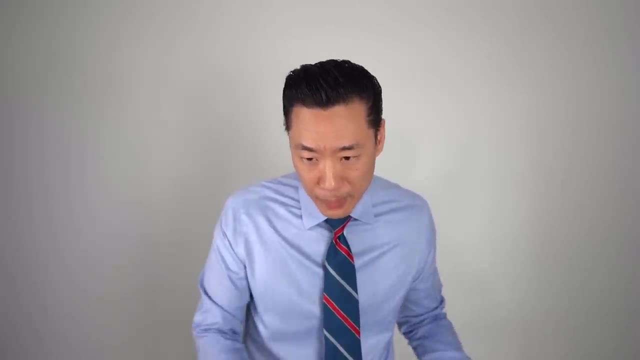 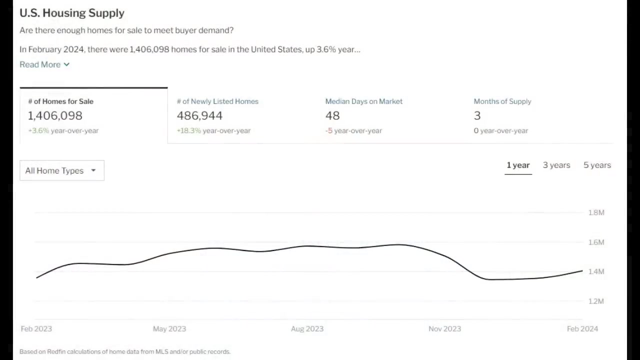 the consequences will be Okay. let's move on to housing inventory. This is important because home prices are determined essentially by supply and demand. So let's take a look at supply. This is a one-year chart. There are currently 1.4 million homes listed for sale in the US. As you can see, it's going. 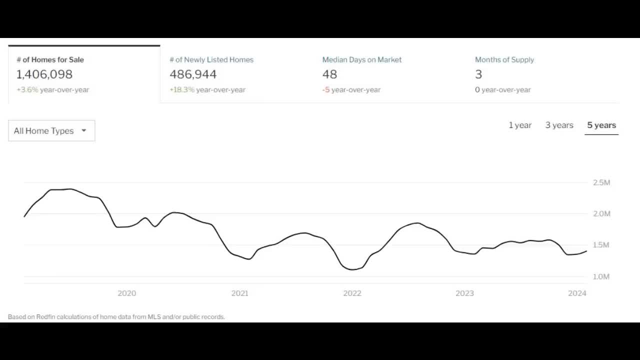 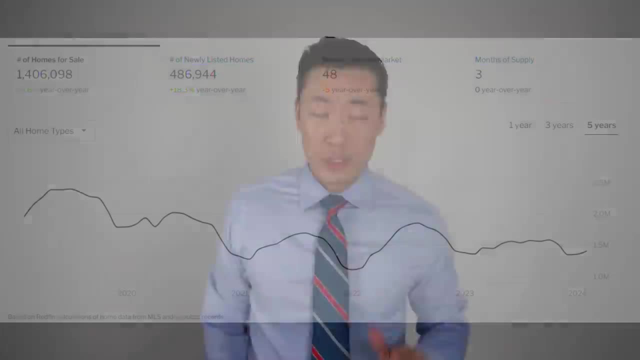 up, but just slightly. So let's zoom out a bit. This is a five-year chart. Look at how many homes were for sale pre-pandemic. So if you look at 2019, it was near 2 million. That's 42% more compared to today. So listen, if you're. rooting for a housing market crash, then this is very bad news, Because if you want a crash to happen, then you want there to be more sellers, More sellers that are trying to get rid of their homes, dump their homes for fire. sale prices: Just sell, sell, sell right, But as you can see from the data, that is not. happening. There are fewer sellers. So listen, if you want a housing market crash, that's great. Sign me up, Let's do it. I'll buy a property, too, with you when there's a housing market crash. But let me know in the comments down below why you think a. housing market crash has not happened yet. Why it's not happening Now? let's talk about mortgage interest rates. Right now, the 30-year fixed is around 7%, So are interest rates going to go up or down in the short term, For the very short term? so I'm talking about April. it's not going to change by much. It's going to be stuck here around 7%. So here's what's going to happen mid-term. So I'm talking about 3 to 4 months. So in the summertime, that's when interest rates should start their sustainable. descent. The reason why I'm saying that is because the Federal Reserve is most likely going to start cutting interest rates this summer, around July. If it's late, then they'll start in September. Once they start cutting interest rates, they're not going to stop, So mortgage interest rates will continue to. decline once they start. Now to be clear, I want to be absolutely clear about this: Mortgage interest rates, when they start going down, they're not going to go down in a perfect, straight, linear line. It's not going to go like that. It's going to go up and down, up and down, but it's going to. go more down than up. So, yes, there's going to be fluctuations. Okay, so how far are mortgage interest rates going to fall By the end of the year? it should be around the 6% range. It could be in the mid to upper 5% range if we're lucky. But the Federal Reserve Plan. 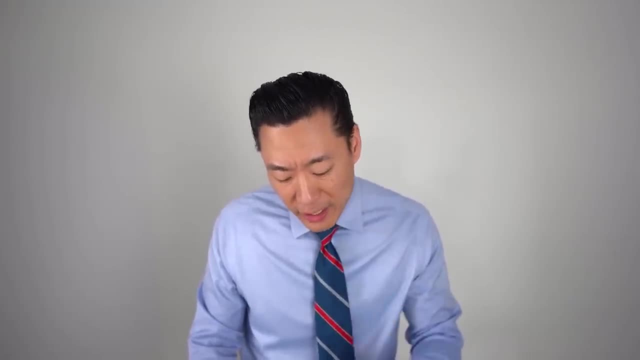 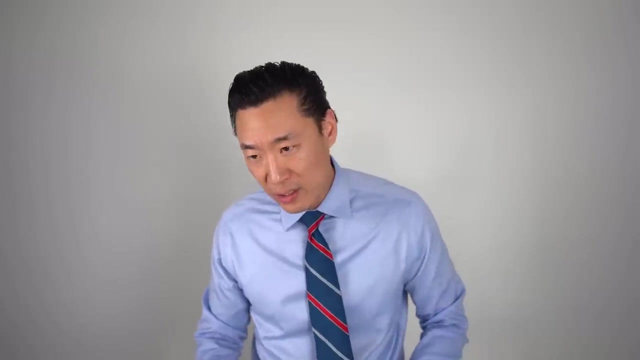 so again, it's public Information- is to continue cutting interest rates in 2025 and 2026.. Therefore, lower interest rates this year. That's just the start. So if you're like, OMG, 6% or 5 point something percent, that's still very high, Well, it's just going to go. lower in 2025 and 2026. At least that's the plan- And at that time you could refinance- A lot of people can't. But, as we discussed, a lower interest rate will add more buying pressure. Now I want to clarify. this: Okay. lower interest rates will add more buying pressure, right? That does not mean that home prices are guaranteed to shoot up. No, it just means that lower interest rates add more buying pressure. So I want to explain. So I'll say it like this: Let's say the interest rates go down. okay, If the housing market were to crash by 20%, then if they lower interest rates, then maybe it's going to fall by 10% instead of 20%, Because the additional buying pressure would prevent a deeper decline. And on the flip side, let's just say the home prices. they're going to go up by 3%. But if they lower interest rates, then maybe home prices will go up by 10% rather than 3% because of the additional buying pressure. Now I want to show you this. You're looking at the number of homes sold, So this is a five year. 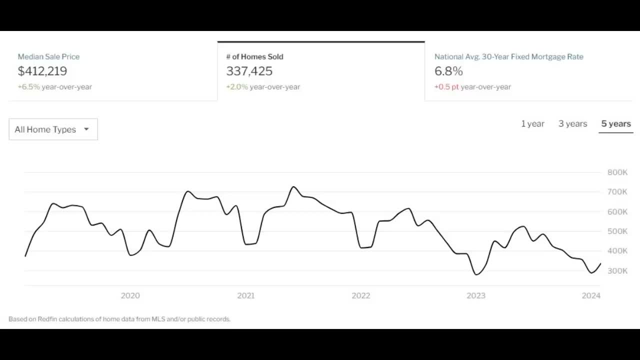 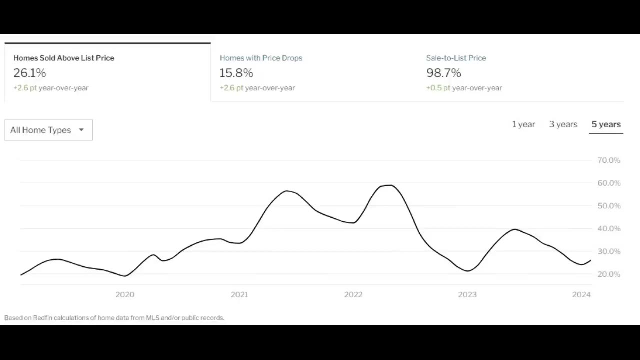 chart. As you can see, it's at depressed levels. So that's what happens when home prices shoot up with higher interest rates. So homes are less affordable and fewer homes are being sold. Now I want you to look at this five year chart, And this is good news for buyers. So this shows. 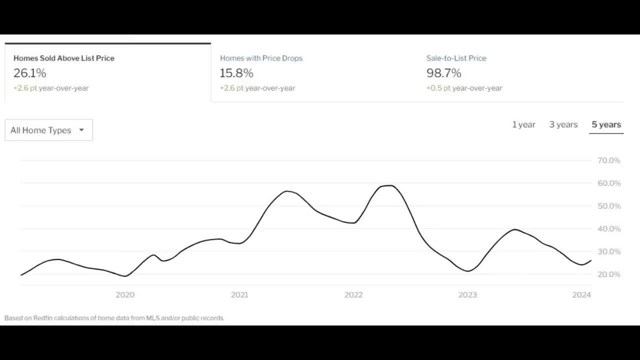 the percentage of homes that are selling above list price. Twenty percent, 26.1% of homes are selling above list. So we are back in the normal range. So that's good to see. It's at the high end of normal. 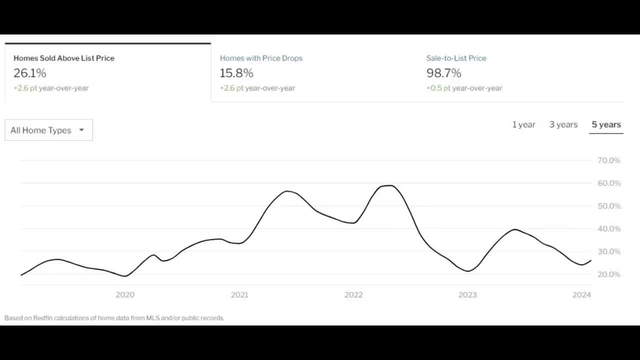 but at least it's nowhere close to as bad as it was in 2021 or 2022, right, But keep in mind. so keep this in mind, because if you're buying a home right now, I don't want you to overpay for a home. 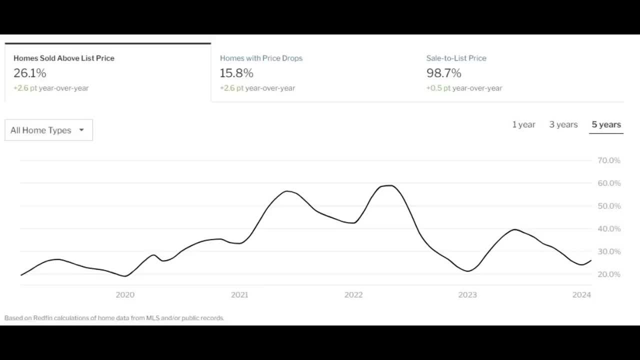 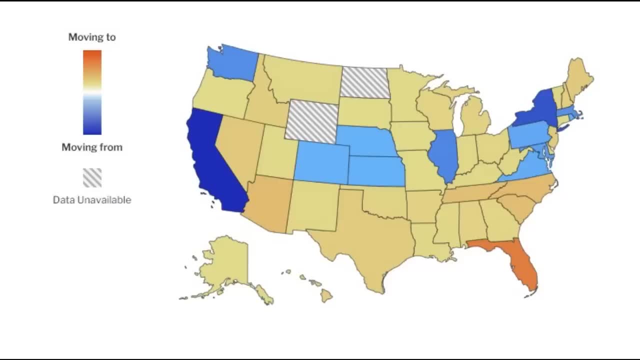 But the reality is that one out of every four homes is still selling above list price. And here's the migration chart from Redfin. This shows us where people are leaving and where they're going. There's still a lot of outflow from California- New York. 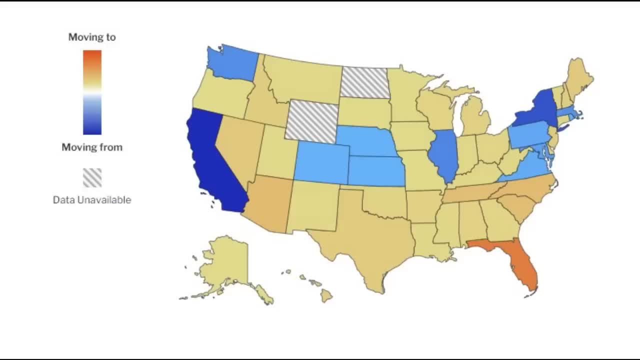 My state of Illinois is in third place, Washington is a close fourth. Florida is still the number one destination. Migration to Texas has slowed down. a lot More people are going to Arizona, Nevada, Tennessee, North Carolina, South Carolina, among other states. 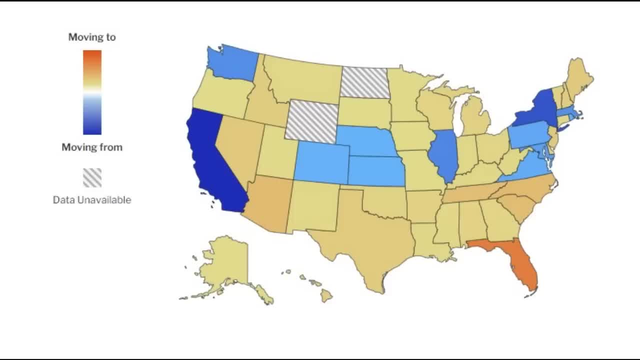 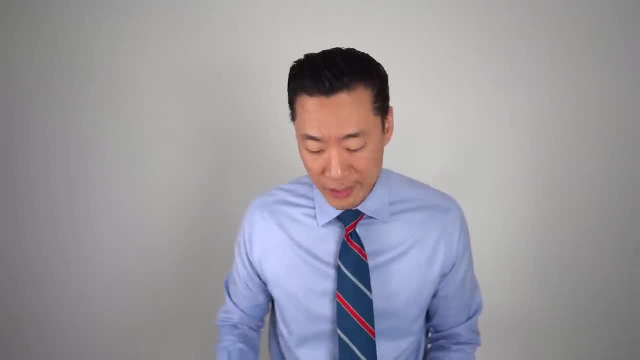 Just to be clear, there's still a net inflow to Texas, but it's slowed down considerably. Now let me tell you about home prices this year. We're talking about forecasts, So the big institutions are predicting it's a range. It's a drop of 2% to an increase of 5%. So the predictions, depending on the institution, they're all over the place, but they're mostly in that range. So nothing drastic, no housing market crash, but then again no housing.